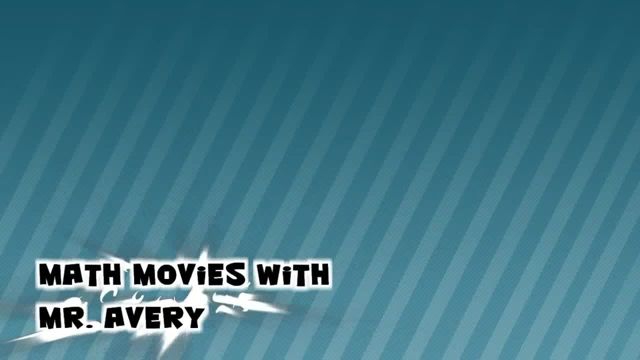 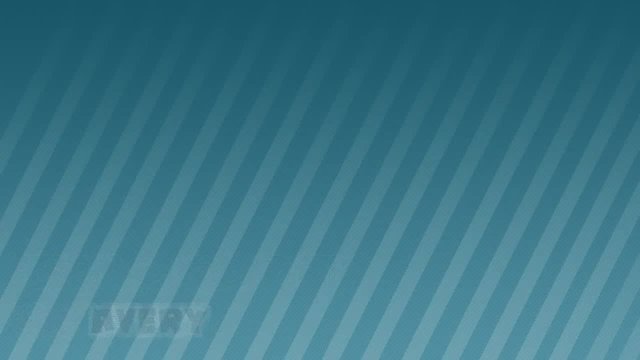 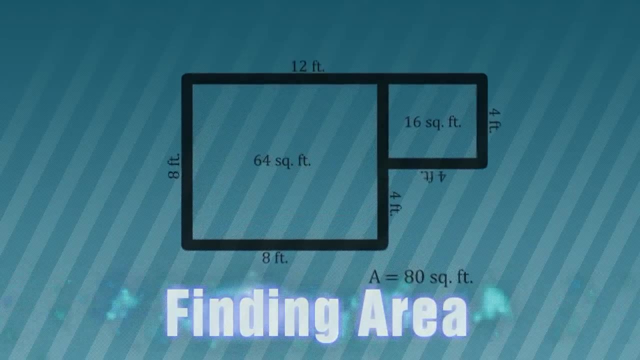 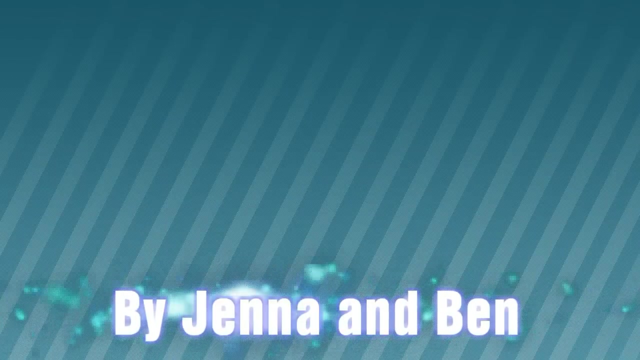 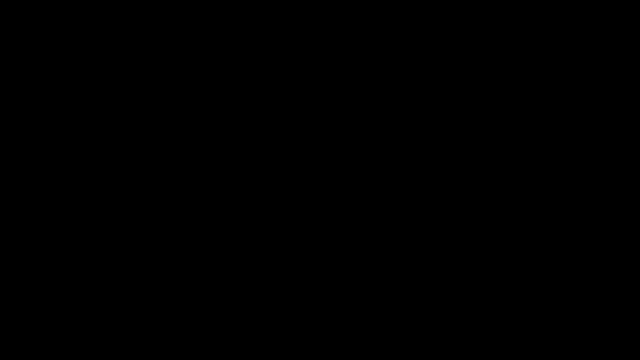 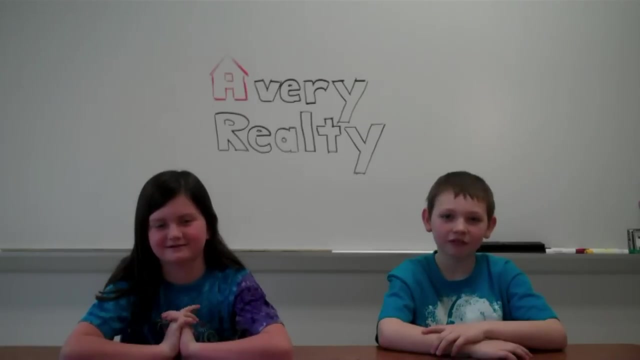 Thank you for watching. Hi, I'm Beth, Hi I'm Jagger, and we're here with the Avery Realty. We're going to show you how to find the area of a room. You find the area by multiplying the length times the width of a rectangle. 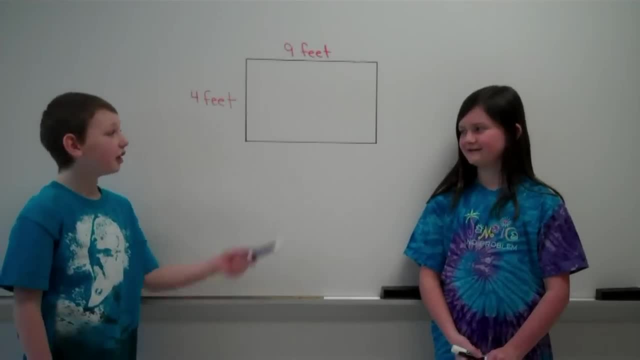 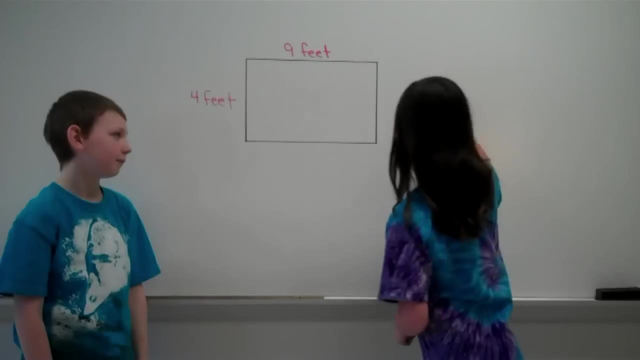 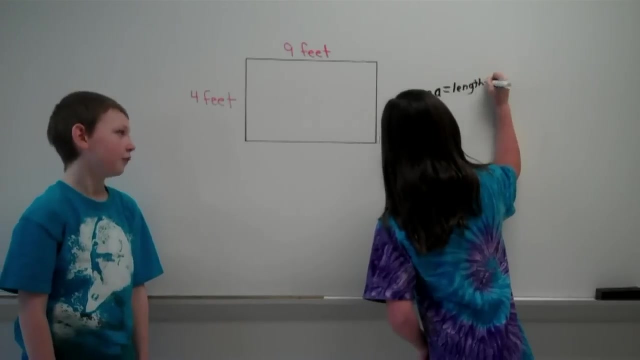 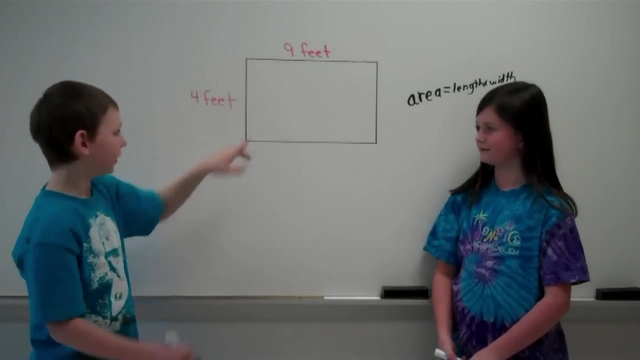 Now let's go to the board. Today we're going to show you how to find the area of a rectangular room. In order to find the area of a rectangular room, you have to multiply the length times the width. So we have 9 feet times 4 feet. 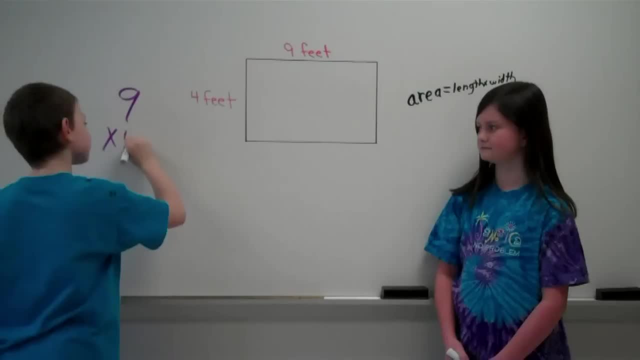 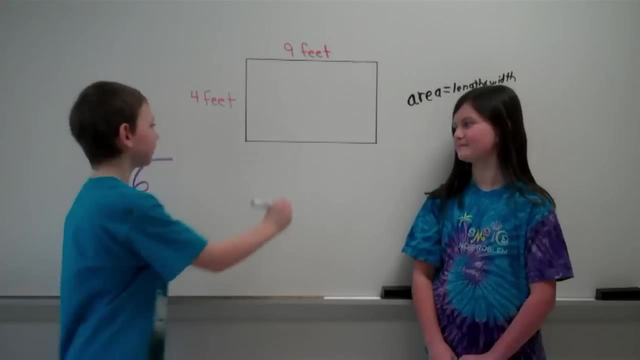 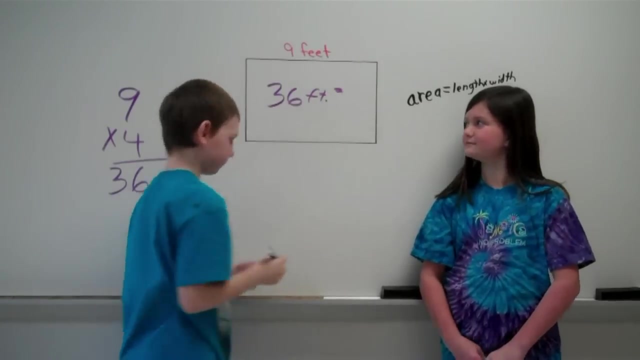 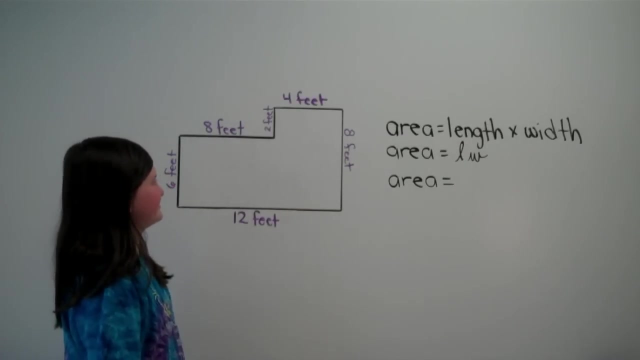 So that is 9 times 4 equals 36.. So our answer is 36 square feet. Here's the next round. We're going to find out how to get the area of a regular shape room. First, you have to break it up into different rectangles. 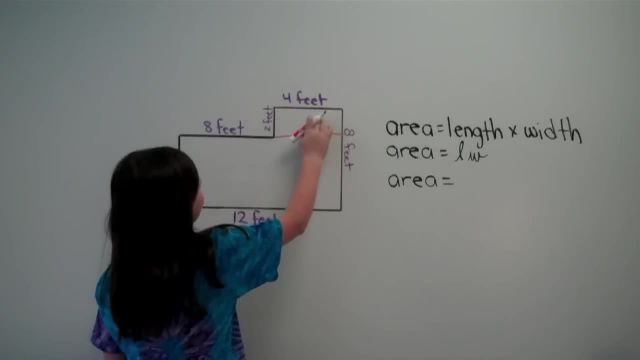 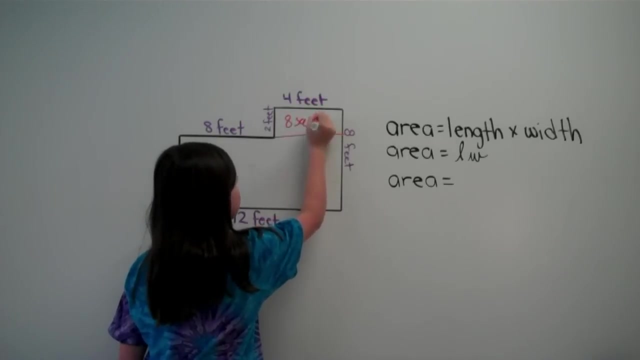 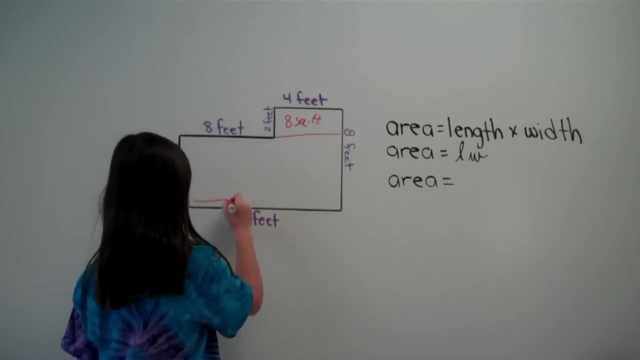 Then you would multiply the length, which is 4 feet, and the width, which is 2 feet. which is 4 times 2 equals 8 square feet, And then you would have to do this rectangle which the length is 12 feet. 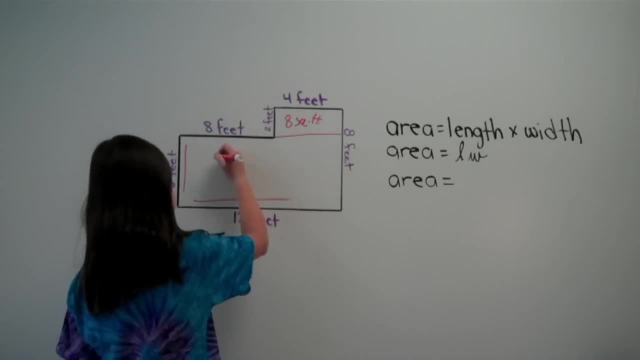 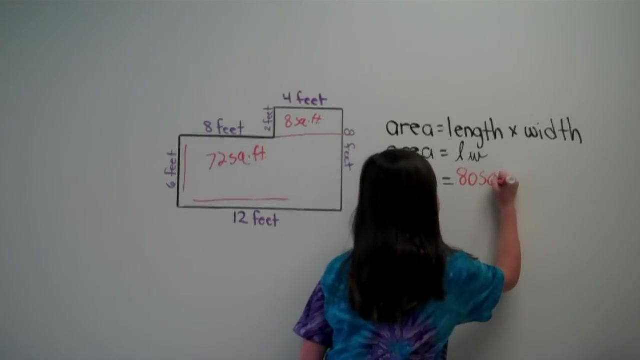 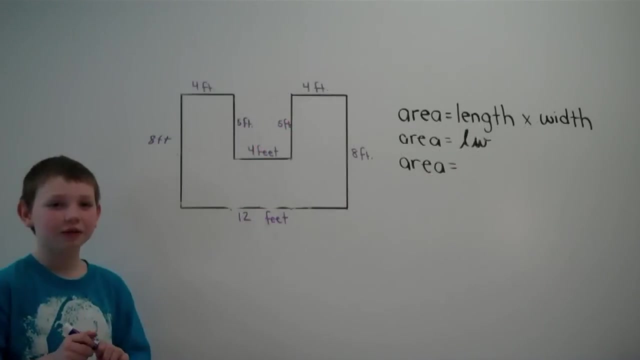 and the width is 6 feet. So you would have to do: 6 times 12 equals 72 square feet. You would have to add them up, which 72 plus 8 equals 80 square feet. Thanks, Jenna. Now let's show you the last one of the house.